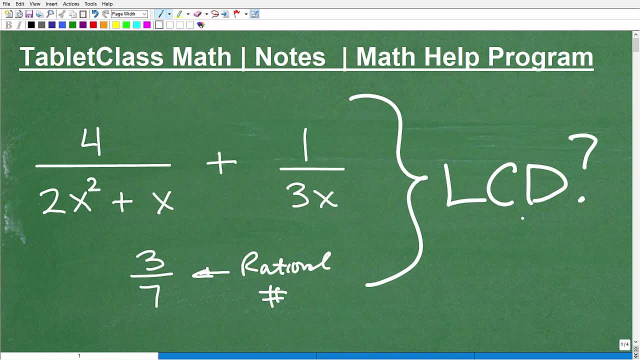 fractions is understanding how to determine the LCD. So before I get into all of this, first let me introduce myself. My name is John. I'm the founder of Tablet Class Math. I'm also a middle and high school math teacher And over many, many years I've constructed 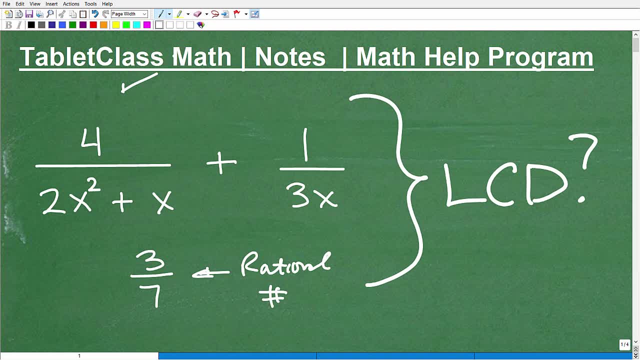 a ton of observations. I teach online math courses. These are super high quality, fully comprehensive math courses at the middle and high school math level. So if you need a math course, okay, if you're looking to take one online. or you need a program to help you with your current math. 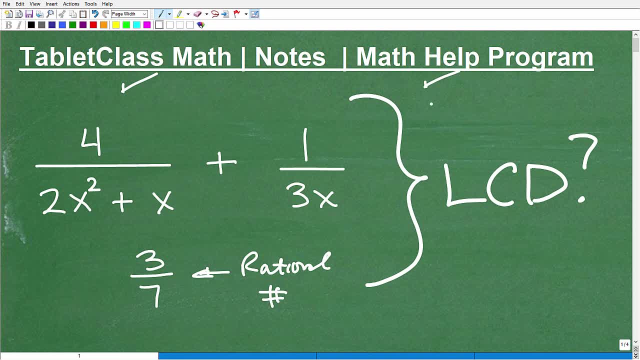 course I'm going to leave a link to my program in the description of this video. That's my full instruction. I probably have, you know, I'm just not good at math. I'm not good at math, I'm not exaggerating, But I probably have the most videos of any program that I know of. 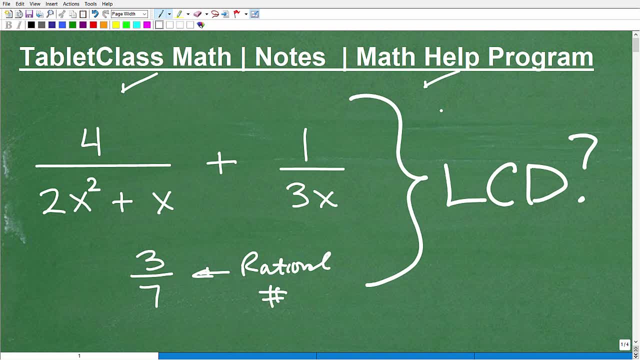 online. It's taken me well over a decade to build out all my content on here, And I've done it to make sure you get everything you possibly could need at these various math levels. Okay, there's a lot that goes into not just doing it like I'm going to do a quick tutorial video here. But if 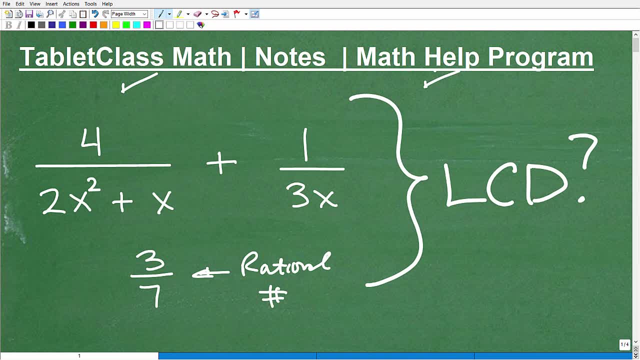 you really want to master math, you need complete, full instruction and a ton of example problems that are being solved. I'm going to leave a link to various math notes that you might be interested in: pre algebra, algebra one, algebra two, trigonometry and geometry. This LCD stuff here is generally 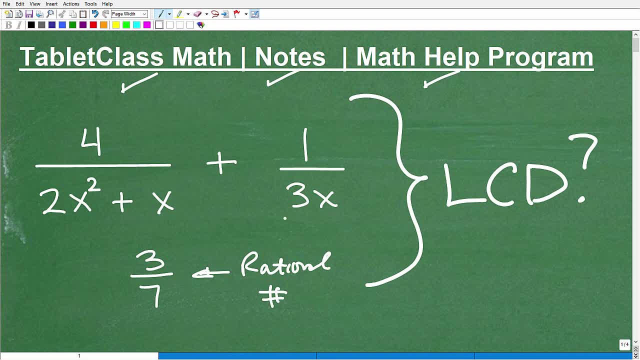 taught kind of really get into it at the algebra one level. So it's kind of introduced at the pre algebra level. So if you don't have a good pair of notes on this and you want a good pair of notes, you know where to find those as well. Okay, so let's get into. 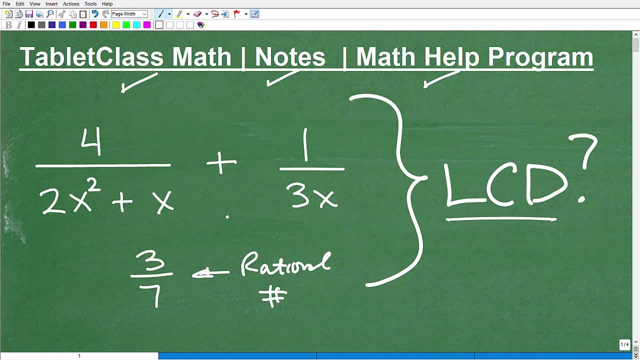 finding the LCD the lowest common denominator for a problem like this. So here we have a fraction, right Variable fraction. we call these rational expressions And we want to add them up. this would be no different than say, taking this fraction three tenths plus one 15th. Okay, 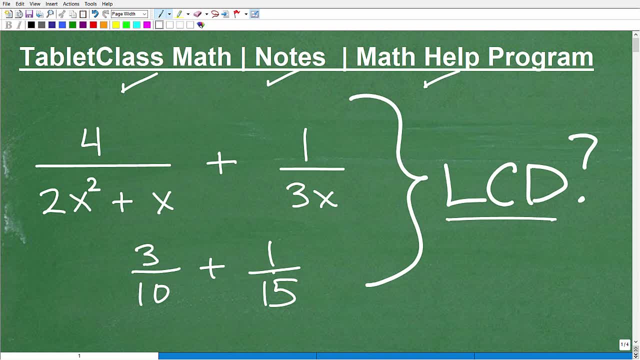 and I'm going to add these two fractions up. By the way, I just did a video on how to find the LCD with fractions where the lowest common denominators were only numbers. So if you don't know how to find the LCD where the denominators are only numbers, 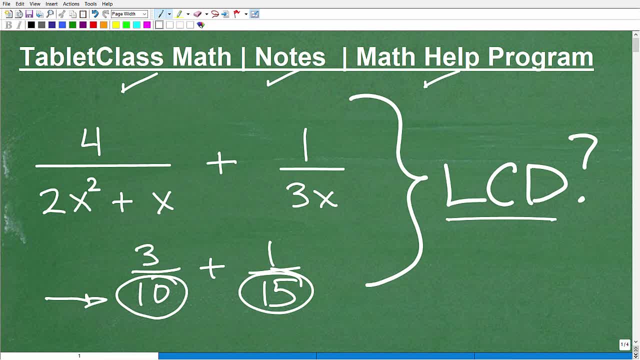 okay, then you want to review that. I really shouldn't link it to this here video, But if you, if you go into my playlist, you'll- you'll find it in the pre algebra playlist or somewhere on my channel if you want to learn this. but you got to know how to do. 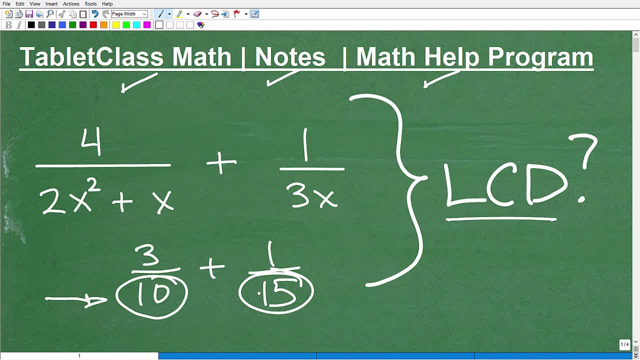 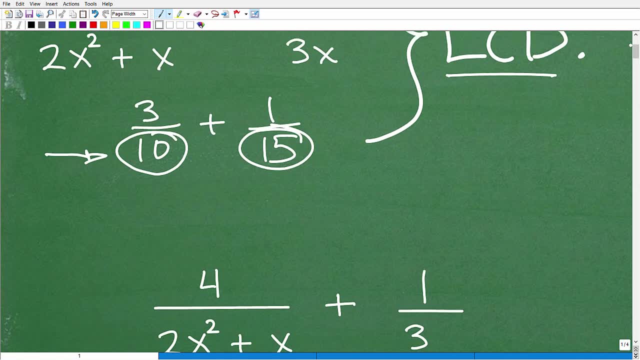 this first. Okay, now, here you know, finding the LCD of 10 and 15.. Let's just review that real quick. Okay, you should already know how to do this, you should be an expert in it. But what we're going to do is what this is. five times two, that's the factors of 10.. And this: 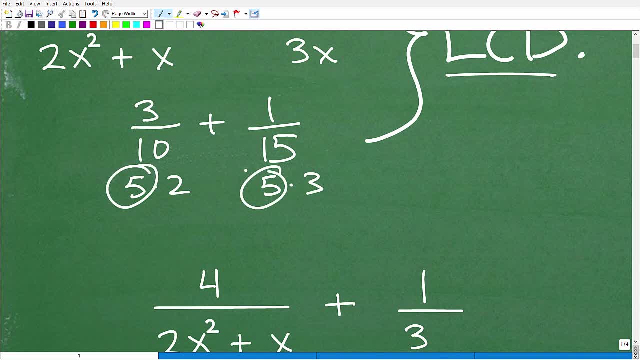 is five times three. So we need- these are the prime factors- we're going to need a five, And then we're also going to need a two and a three. So that's two and three and we multiply all these together, that's 10 times three, it's 30.. Okay, so the LCD. 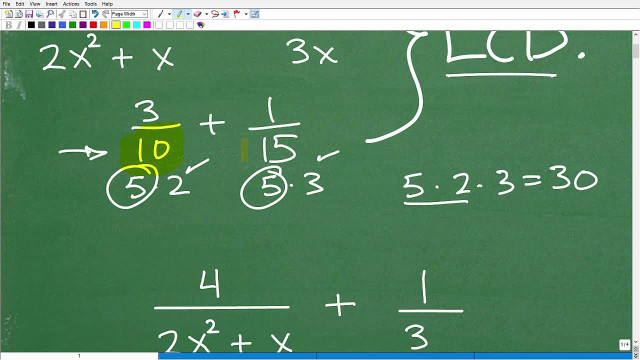 here. okay, in this particular problem with 10 and 15, as our denominator is 30. And we were able to do that because we looked at the prime factors and we selected each one of, or we needed each one of, these prime factors represented in a product. Okay so five is a prime factor, two and three, all these are the unique prime factors in the denominator and we multiply them together, we get our LCD. Okay so, 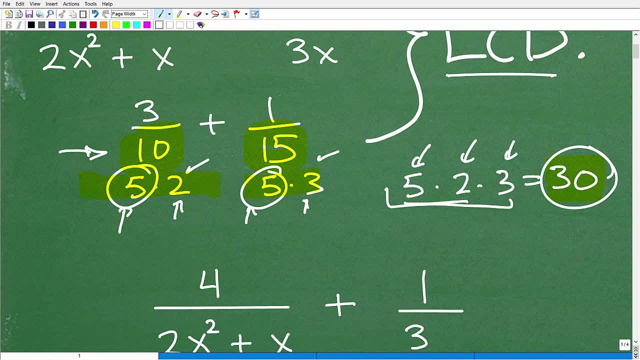 that's how you find the LCD technically. Now most of you would. you know, way back in the good old days, and you know sixth grade, fifth grade, you'd be like, Oh yeah, what's the lowest number? you can just look at this problem, kind of figure it out like, Oh yeah, 30, 10 goes into 30,, 15 goes into 30. And that's fine, you know to do that. But when you have larger values you need a more. you know technical procedure to find the LCD And this is what it is Okay. so you got to, you know, hopefully understand that And 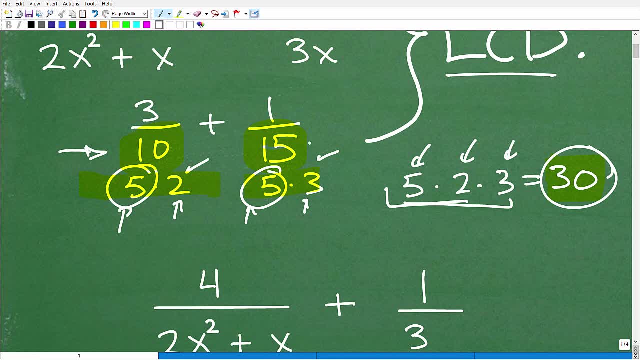 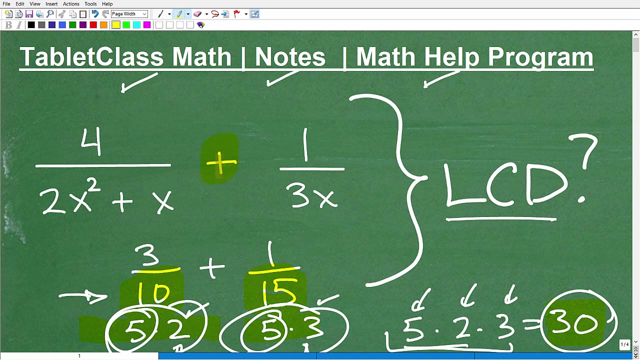 strengthen your understanding of working with LCD. when it comes just to arithmetic, Okay, but what was the key here? the key was factoring. All right, And I stress this in many of my other videos- is that what you learn in arithmetic carries over to algebra, Okay. So, again, when we look at a problem like this- excuse me, what am I trying to do? I'm trying to add two fractions, Okay, so I can't add these two fractions unless the denominator 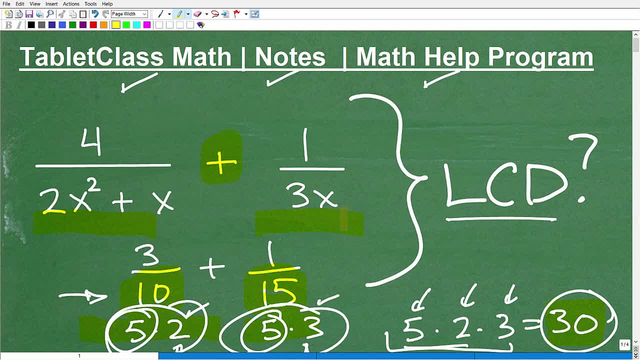 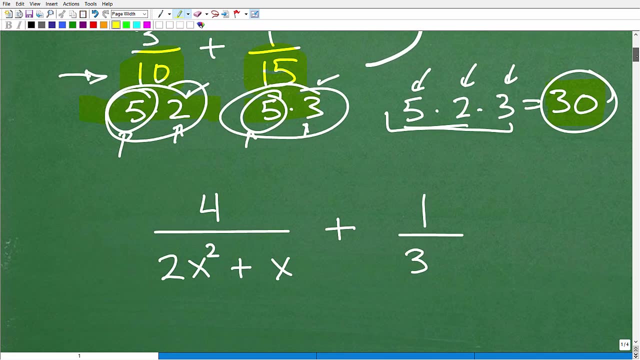 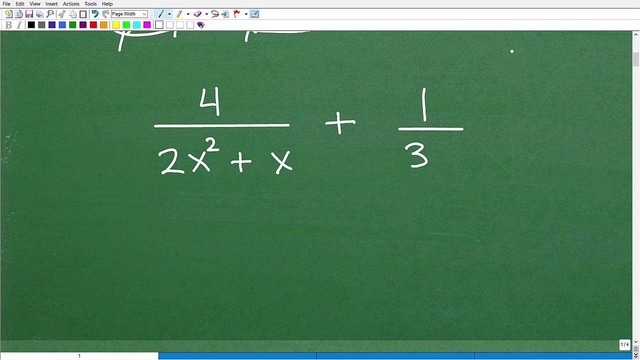 are the same. Okay, so I need to rewrite these fractions And in order to do that, I need the lowest common denominator. right now I'm not going to get into how to to complete the pool, the full problem, Okay, because that's kind of distract away. I'll do other videos on that. Right now, I just want to keep the focus on finding the LCD, because this is a place where a lot of students get confused, So let's just focus on LCD. 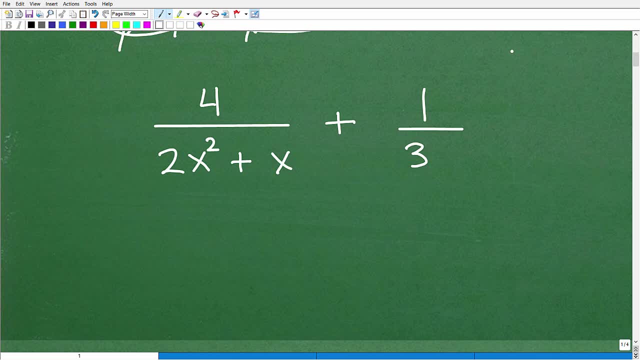 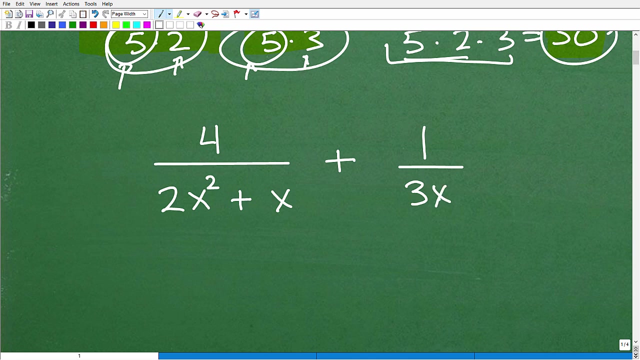 Again, if you need more math help with this topic for adding or subtracting rational expressions, you know where to find that And I'll do more future videos on it. That's why you want- definitely want- to subscribe to my channel. All right, so let's get to this problem. So we have four over two x squared, plus x plus one. I think we had an x here. Yeah, one over three x. Okay, so here is our problem. So what are the skills that we're going to need here to solve or find? 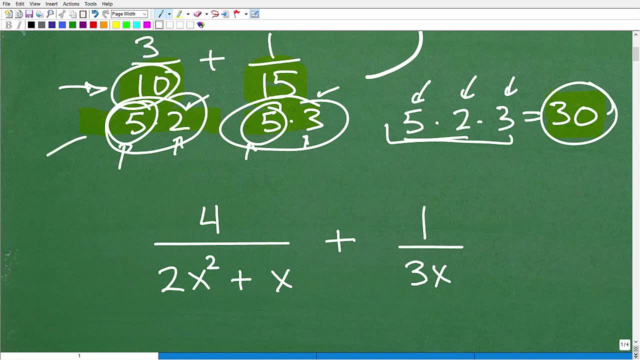 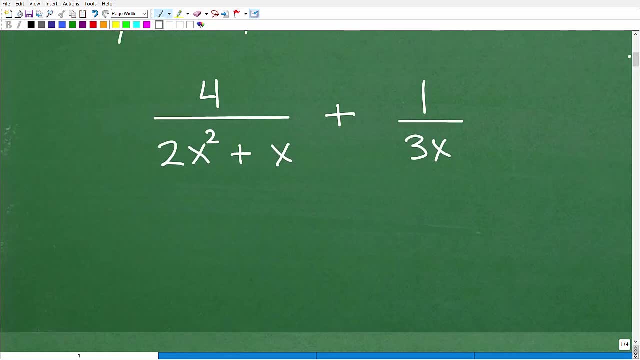 the LCD. Okay, well, just like over here, you know, I factor 10, and I factor 15, you need to know how to factor. you need to know how to factor. So in algebra I stress this big time in all my courses- but factoring is a critical skill. If you can't factor, you're not going to be able to add, subtract, rational expressions, just you're not gonna be able to do a ton of things. So you got to make sure you have good factoring skills. If your factoring skills are weak, then that's a whole separate topic. Okay, and that's a pretty big 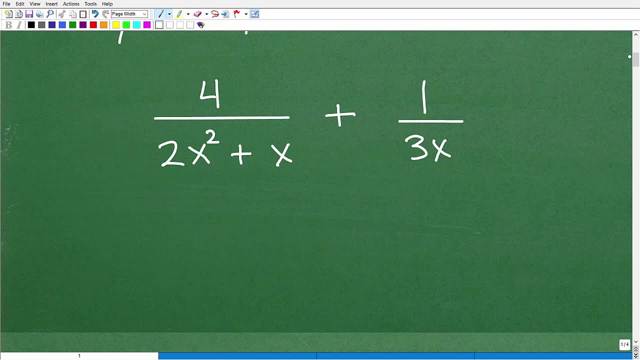 discussion. discussion in and of itself, But let's go ahead and see if you can factor. if you want to kind of follow along in this video, I would pause the video and factor, factor this expression And then just think about what, what the factors of this expression is right here? Okay, All right, So this expression, this right here, this denominator, I can factor out an x, So this would be x times what, that would be two x plus one. 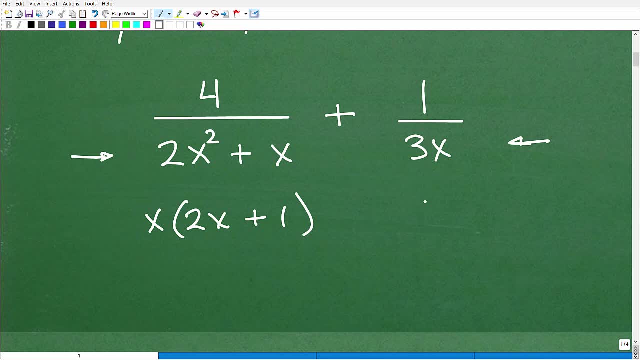 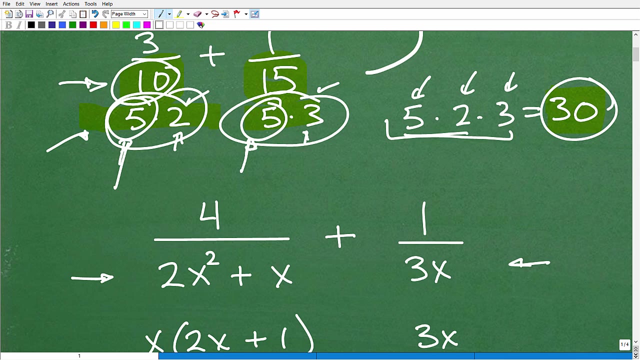 So if you got that right, that's excellent. And then this is basically just three, x. Okay, that's the factors three and x. Okay, so now let's follow kind of the pattern of what we did over here. Okay, so once we got everything factored, each unique factor had to be represented. unique prime factor had to be represented in a product for LCD. Okay, so let's go ahead and build out the LCD here. 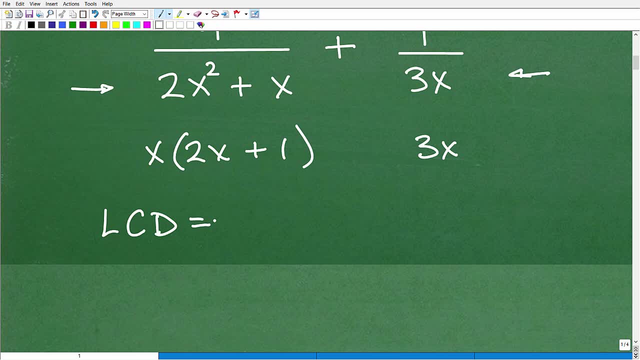 LCD. So what is LCD? Okay, so I have x. okay, I have an x as a factor. Okay, this is this. these two things are factors. Okay, Okay, this is two factors. This is x, And then this whole thing here is a factor. Okay, Three is a factor and x is a factor. All right, So you got to make sure you understand that. So let's take a look at this first factor, x. Okay, All right, I have an x here, So that's going to have to be in my LCD. 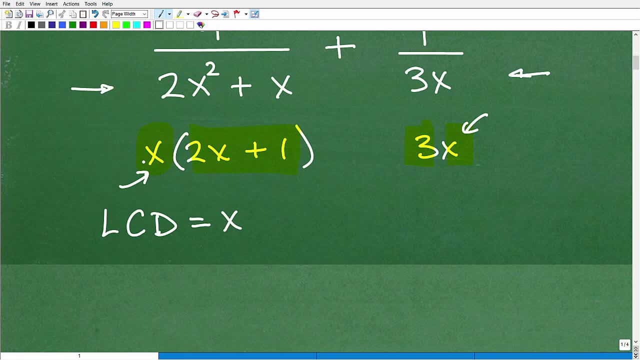 And I have this other x. All I need to do is represent one power of the factor. Okay, so I have an x here and x here. I just need to represent it one time in my LCD. Okay, then I have this two x plus one. All right, I'm going to have to have that in my LCD, because that's a unique factor, And then I have to have my three in my LCD as well. Okay, so what I can do now is: 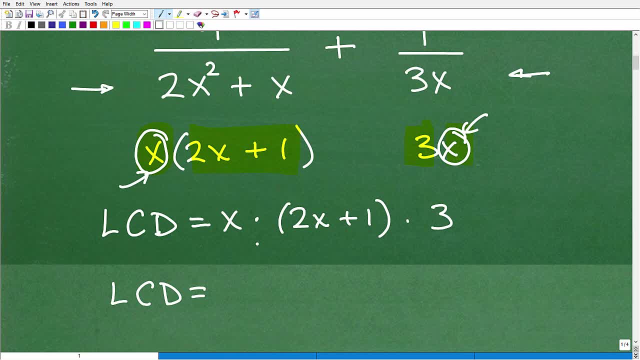 just multiply all this stuff together. So let's do it this way: Three times x, that's three x, and then we can multiply by two x plus one, And when I multiply, this could be six x squared plus three x. that would be my lowest common denominator. Now here's a bit of a tip for you. Okay, when you're actually doing problems involving LCD with variable expression, these rational expressions leave your LCD factor, Okay. so 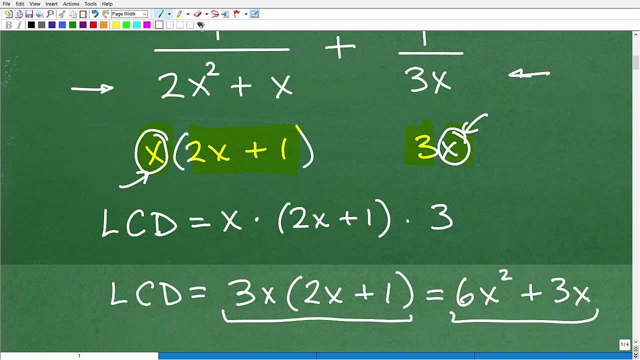 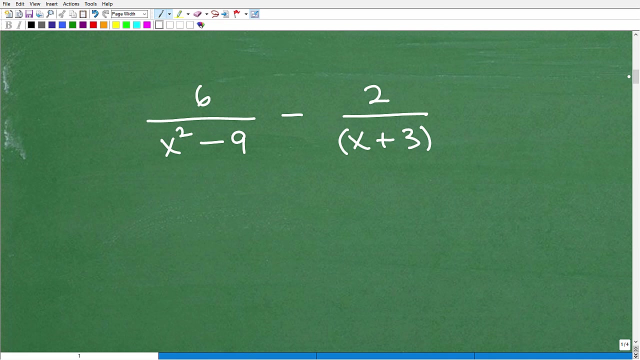 don't multiply back in, Okay, unless you're kind of told to do so, Or if you think that the final version of your answer requires you to do that, Okay, just leave things factor, because that's what's going to benefit you, Okay, All right, So that's a quick example. Let's take a look at another example. Okay, And I can come up with a lot of different type of variations of this. Okay, we can be. I don't want to make this video too long, So I may not cover every single kind of 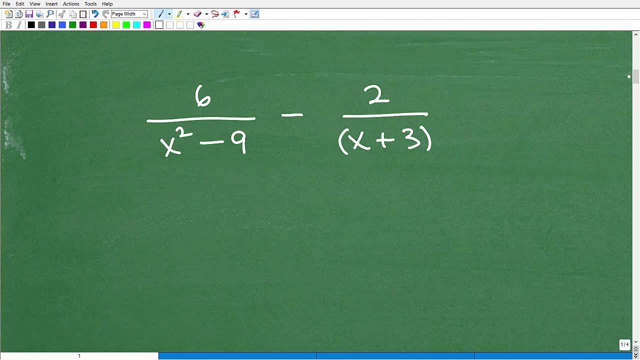 variation of factoring and whatnot, for you to get really, really good at this. Okay, this is just a kind of a quick tutorial to kind of- if you were totally lost in it- for get you on the right path. So you want to practice this stuff, either, obviously, with whatever material you're learning in school or, you know, follow on instruction and maybe some of my other YouTube videos, or definitely my full math learning program. Okay, because this is a fairly involved topic. Okay, so we're just kind of, you know, doing an overview of this. 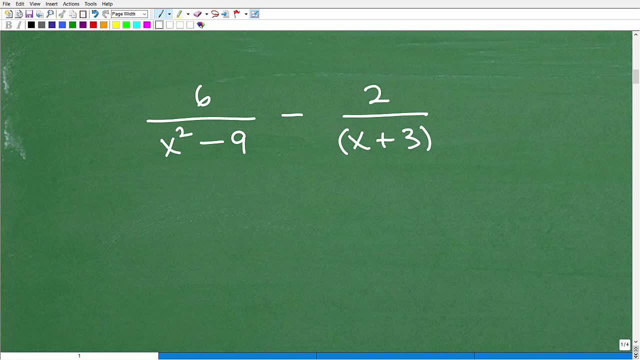 Okay. so we're just kind of you know, doing an overview of this. Okay, so we're just kind of you know, doing an overview of this. I'm looking at the denominators. I'm like, okay, what's the first thing I need to do? All right, So if I want the LCD, the first thing you need to do is got to completely factor each respective denominator. Okay, so again comes back to your factoring ability And go ahead and pause the video if you want to go in and see how strong you are factoring. Can you factor this, these denominators? Okay, so x squared minus nine has the denominator. 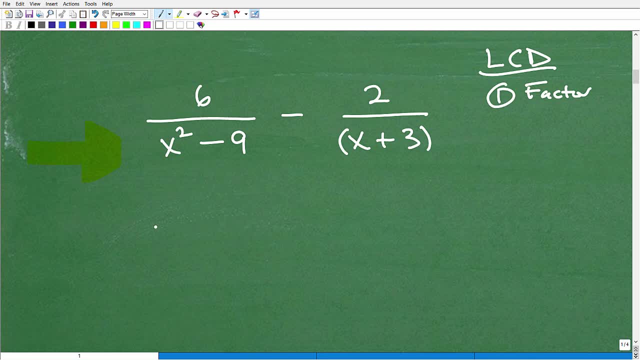 happens to be a factor. Let's just do it this way: As x plus three times x minus three, this is what we call the difference of two squares. So you got to know how to do that, right? So if you didn't know that this was equal to this, then you can't do this problem. Okay, and then x plus three is is just x plus three. that's its only factor one in that. So here is our factors. Okay, so we have this factor. this is a factor. this is another factor of this. 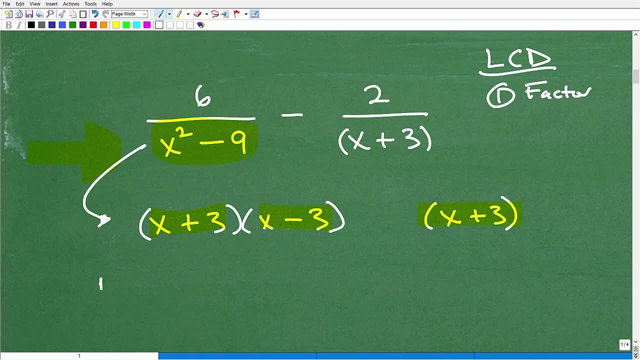 Okay, and this is another factor. Okay, so can you tell me what the LCD is? Okay, what is the LCD? All right, so let's go through this Again. we're going to have to have each factor represented. So I have an x plus three and x plus three and x minus three. So I'm definitely going to have to have an x plus three in my LCD. So it's represented here And it's represented over there. Okay, So, 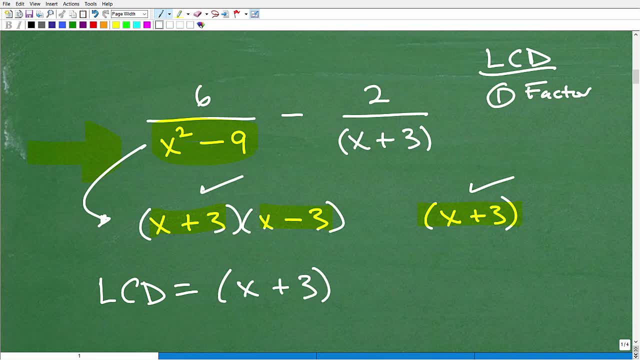 at this point I'm like: well, do I have to write this twice? No, you only have to write the factor once. Okay, as long as the factor is represented one time is fine. And then I have this x minus three. that's also got to be in my LCD, And that's it. This is the LCD of this rational expression. Okay, Now let's kind of mess around with some things here for a second. Let's say I had this scenario. 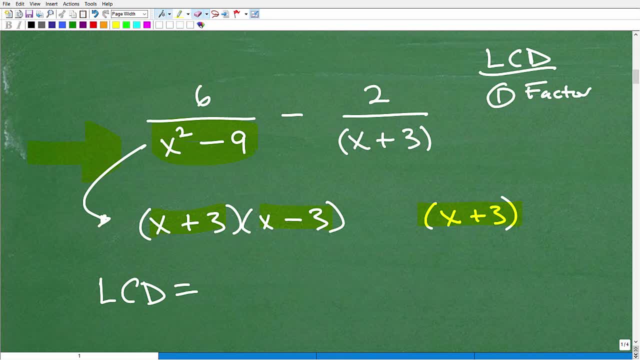 Okay, Let's say I had x plus three cubed and I had this x plus three right here, Okay, So let's say this was my problem. Okay, So what would be the LCD here? Okay, do you think you know what it is? So this is a different type of problem, right? So, x plus three cubed. 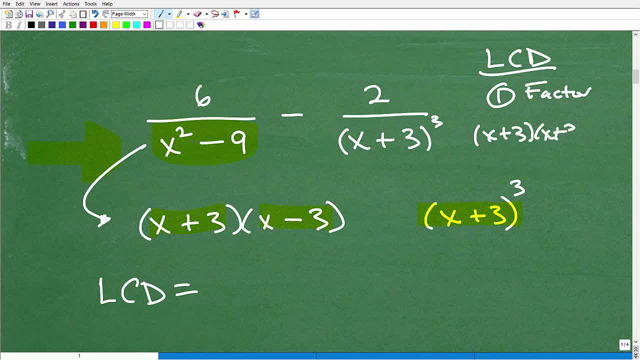 is the same thing as x plus three times x plus three times x plus three x plus 3, right? so we wouldn't write it that way. we would write it as x plus 3 cubed. so we look at these factors. i got- well, i got- x plus 3 here. i got x plus 3 here, so maybe i just need to just 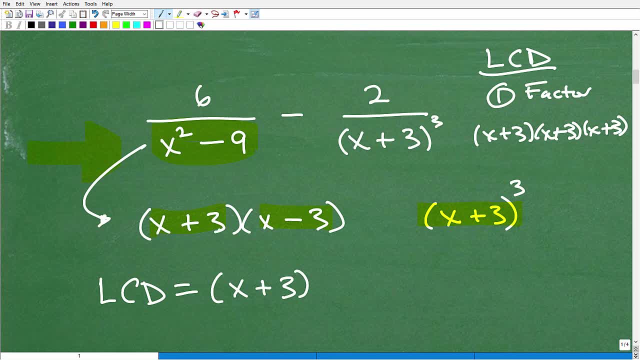 write x plus 3, it's fine. i mean, there's three over here where there's one here. i just need to have it represented. that's not the case. okay, this is x plus 3 to the first power. there's only one of these. this is x plus 3 to the third power. okay, the rule. uh, when you're finding the lcd, okay of. 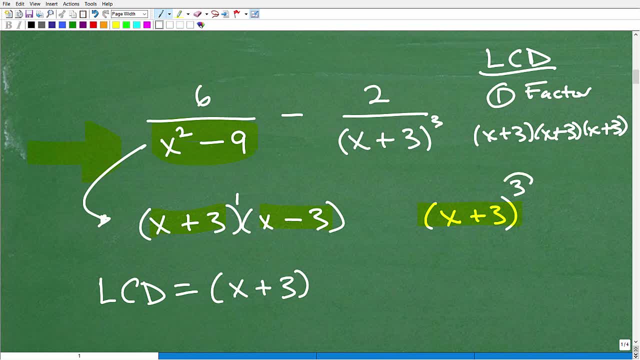 these rational expressions is we have to take the highest power. now this goes to again how to find the lcd of numbers. there's a video i did not too long ago, um, and only in the. i guess a lot of people are struggling this because within a couple weeks that video has already had like close to 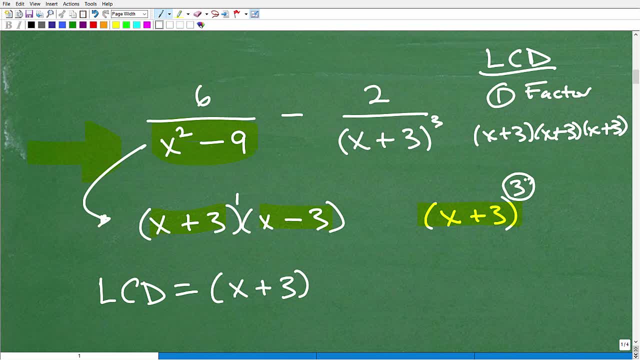 100 000 views. so i'm like, wow, that was that really took off, okay, but that's good. i'm glad that people are like good. getting back to the basics, right, we got to understand the basics here. so we have x plus 3 to the first power. we have x plus 3 to the third power. the rule is: 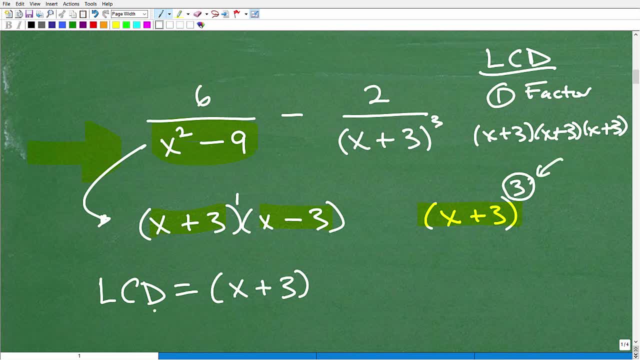 we have to use the highest power, okay, for our lcd. so the highest power of x plus 3. i have x plus 3 to the first, we have x plus 3 to the third. we got to use the highest power for our lcd and then we 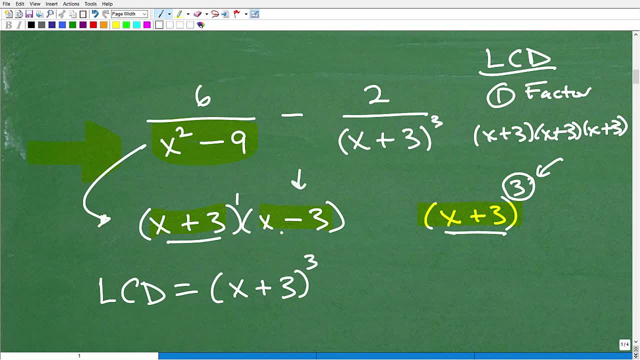 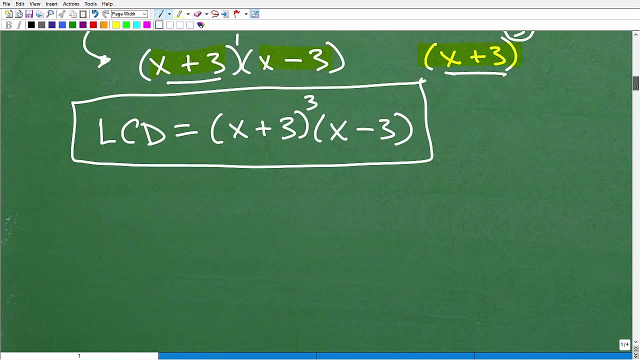 just look at all the other factors and we use the same kind of rule of thumb: okay, oh, i got x minus, that's got to be in my lcd and there is my lcd. okay, so now what we do with the lcd. there's a lot that, uh, you do with the lcd of rational expressions. 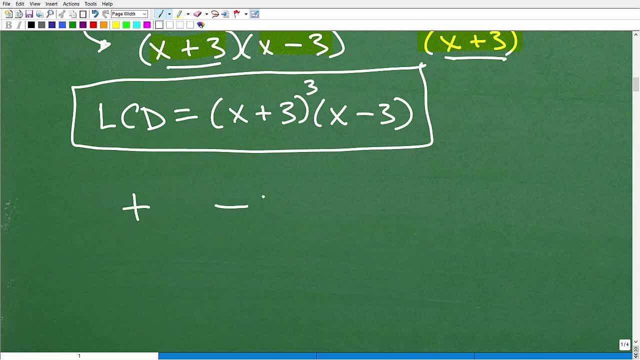 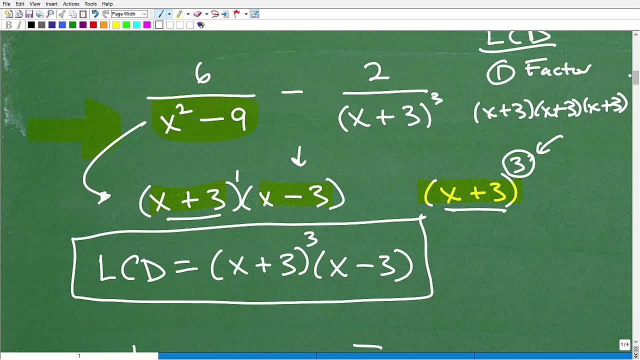 okay, obviously we add and subtract rational expressions, but we also solve rational equations. we need the lcd. the bottom line is you need to understand how to find the lcd of just numeric fractions. okay, uh, one, two. you got to know how to factor, you got to be a factoring. 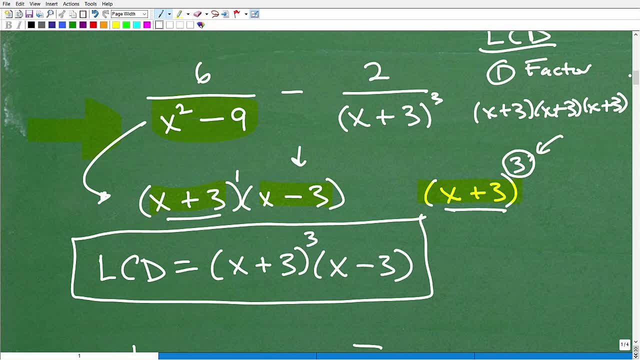 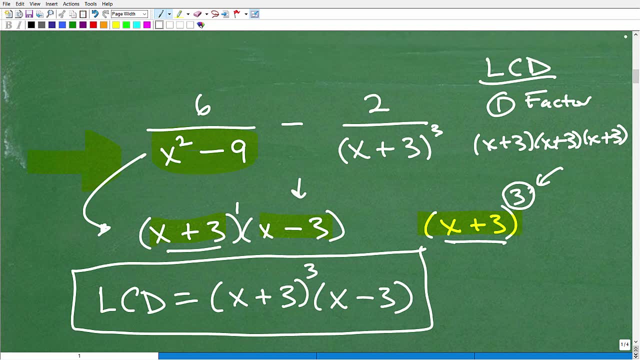 expert. okay, let's go back and review. you know all the things you've learned about uh factoring. the third thing is, once you got all that down, you got to practice how to find the lcd of these rational expressions. just get the correct lcd. once you have the correct lcd, then we can go ahead.